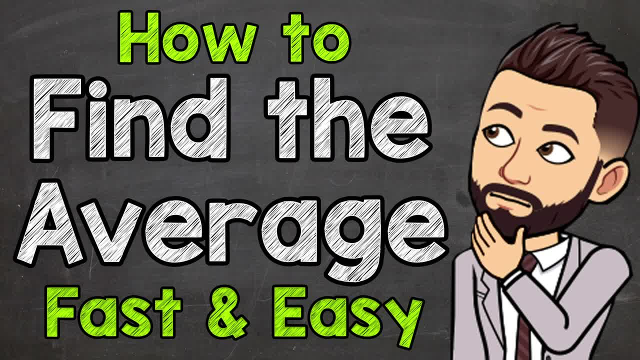 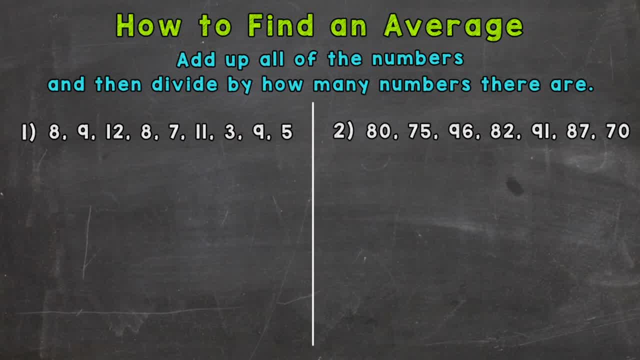 Welcome to Math with Mr J. In this video we're going to discuss how to find or calculate an average, And the average is a number that represents the typical or central value for a data set. Now you see that there are two lists of numbers or data sets on your screen. To the left we have number one and to the right we 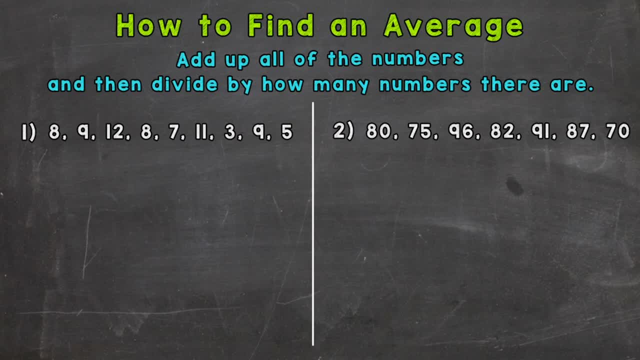 have number two. So we're going to go through and discuss how to find the average for those two. At the top of your screen, in blue, you'll see the steps we're going to take in order to calculate the average. We're going to add up all the numbers and then divide by how many numbers there were. 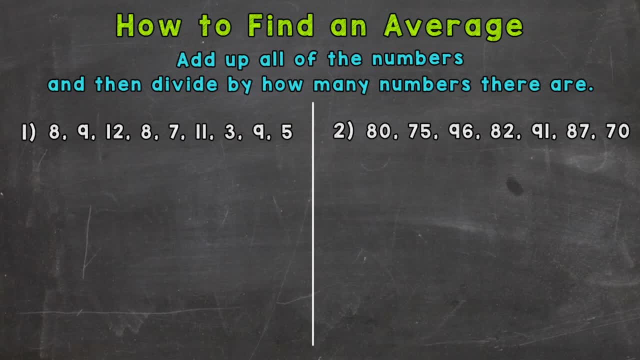 in that data set or list of numbers. So let's jump right in to number one. So for number one, our list of numbers starts with an eight And we actually have a list of nine numbers there. So the first thing we need to do is add up all nine of those numbers. 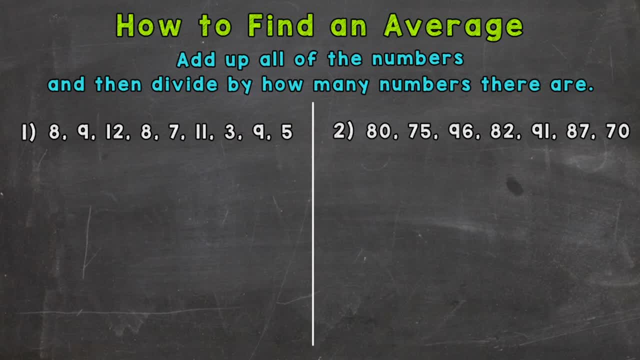 And once we do that we get a sum or answer of 72.. So we again, we added up all nine of those numbers. Once we add them up, we divide by how many numbers are in that list or data set And we have one. 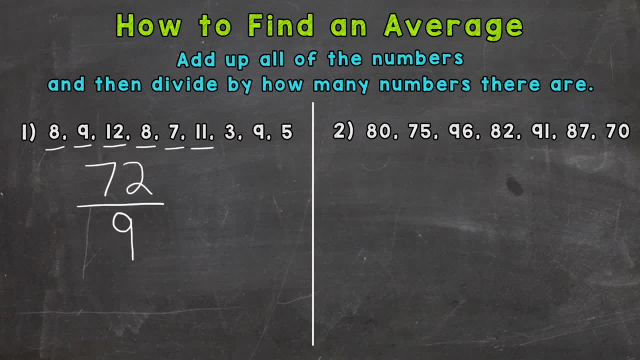 two, three, four, five, six, seven, eight, nine. So we do 72 divided by nine, and that gives us an average of eight. Now it worked out to be a whole number. You will also get decimals when calculating averages. 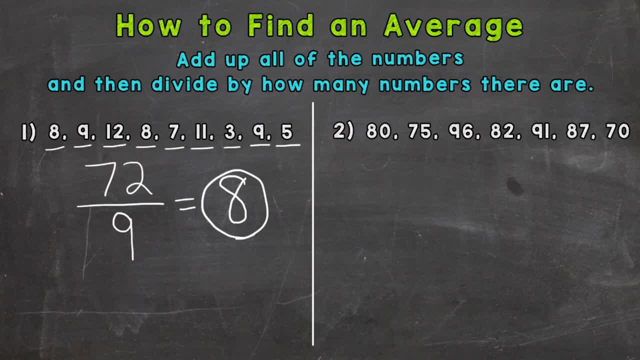 So let's take a look at number two. So we have an 80,, 75,, 96,, 82,, 91,, 87 and a 70. So the first thing we need to do is add up all of those numbers. 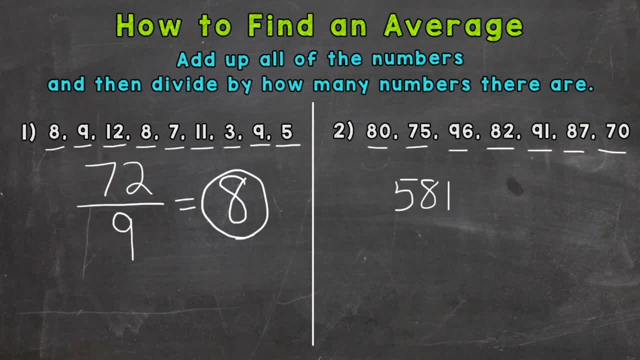 And we get a sum of 581.. Now we need to divide by how many numbers there are: One, two, three, four, five, six, seven. So 580 divided by seven will give us the average, and this one actually turns out to be another whole number, 83 again when. 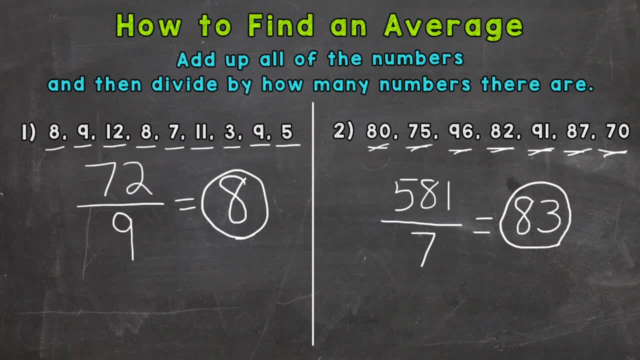 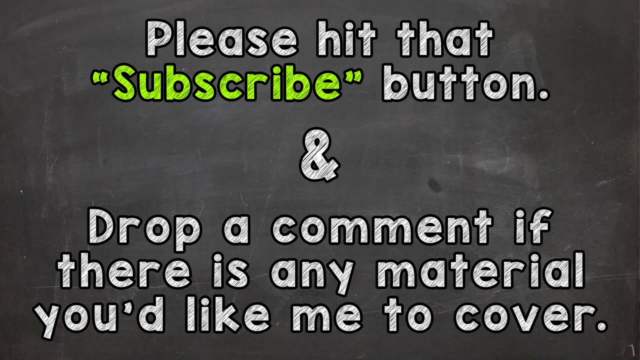 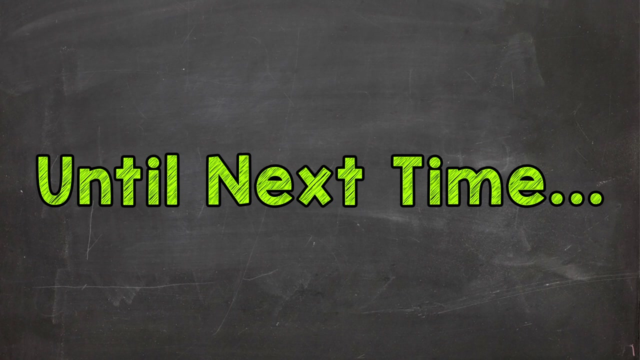 you're calculating averages, you will get decimals. that's okay. so that's how you find or calculate an average. add up all of the numbers and then divide by how many numbers there were. thanks so much for watching. until next time, peace you. 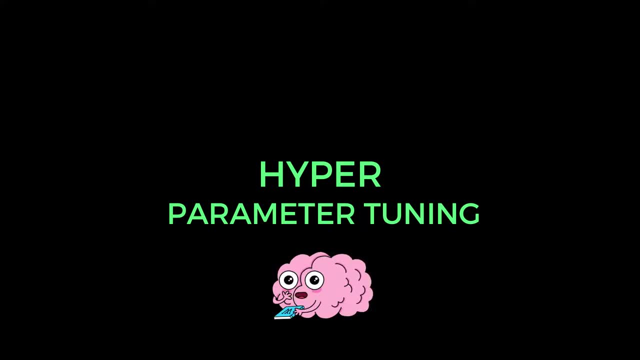 Hello Python programmers, this is AK. In this video I'm going to explain you one of the important method in machine learning that helps you to improve the accuracy of machine learning model. So the concept you're going to see in this video is called hyperparameter tuning. 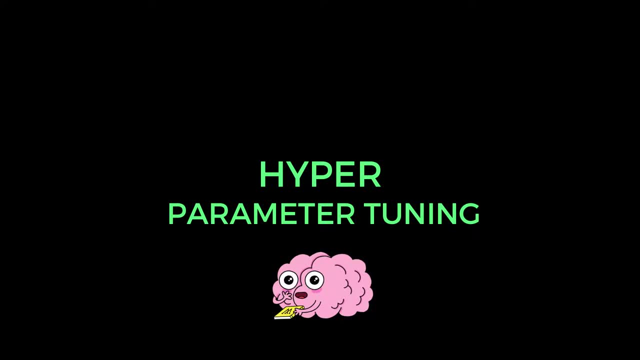 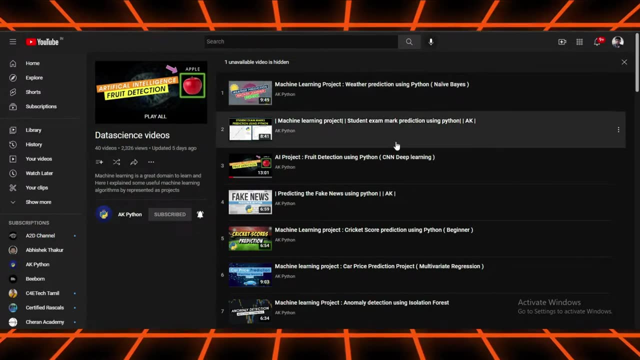 Before starting this video: if you are a beginner in machine learning, then you don't understand this concept. If you want to understand this concept, then please watch my data science videos playlist and learn about how to build the machine learning model from scratch Once you. 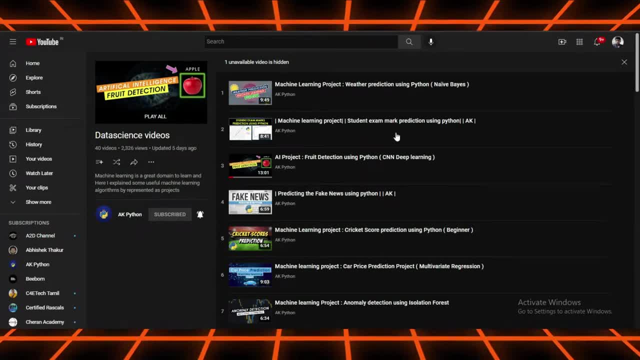 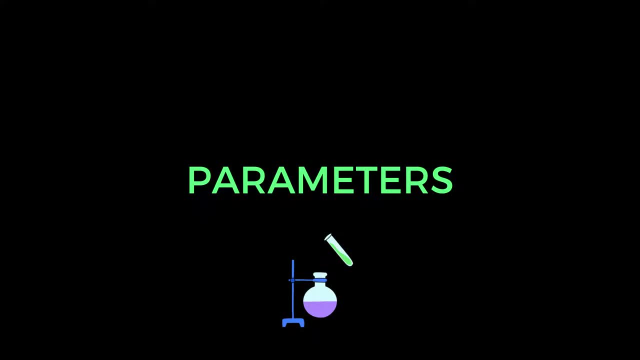 covered up those concepts, then you can easily get to know about what I'm going to speak in this video. Okay, so before you enter into this video, you should definitely know about what is parameters in machine learning model development, Because the hyperparameter tuning concept is entirely. 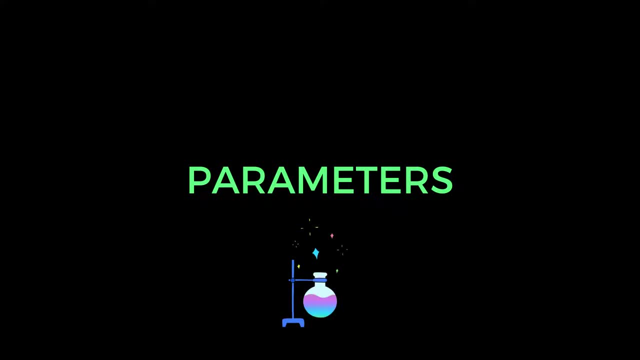 related to parameters in machine learning And also in this video we entirely focus on how to improve the model accuracy using parameter tuning. So I will show you how hyperparameter tuning is improving the model accuracy with some practical examples. Okay for explaining this important. 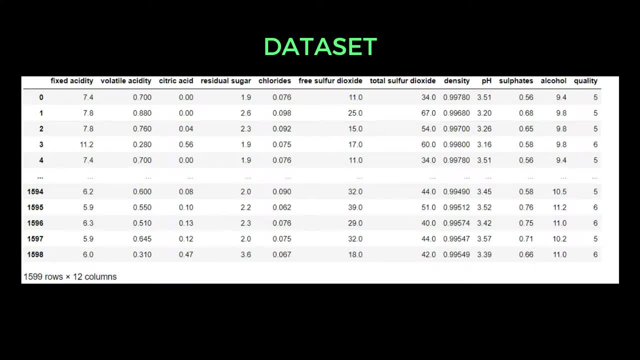 concept. I'm going to explain the concept of hyperparameter tuning. So let's get started. So let's get started. I took one data set called wine quality. I will provide a link for this data set in the description So you can download this data set from there. Okay, Actually, in machine. 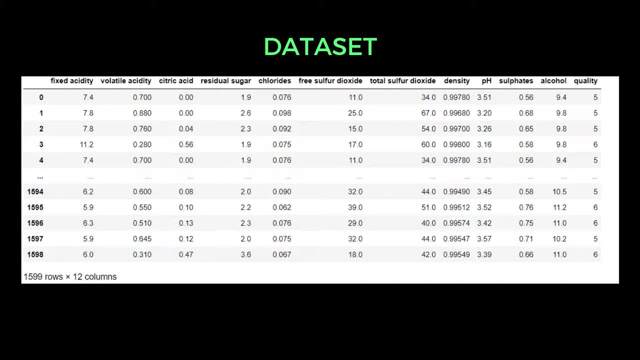 learning. if you're trying to improve the accuracy of ML model, then there are a lot of techniques are there? hyperparameter tuning is one of the technique that will help you to improve the model accuracy, And if you want to know about the rest of the techniques, then I already made a video.